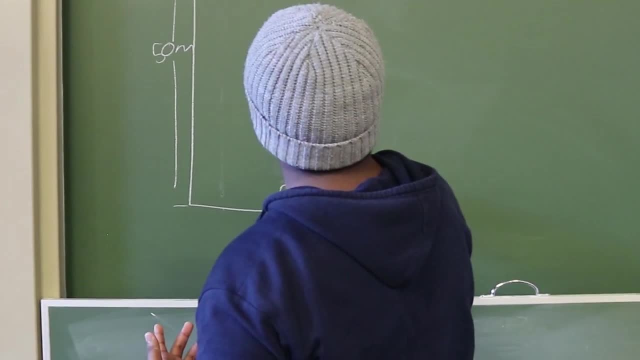 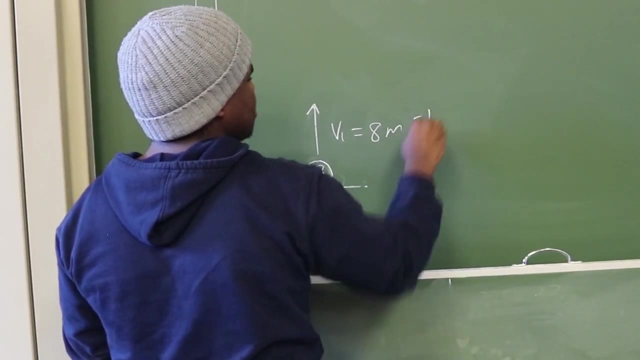 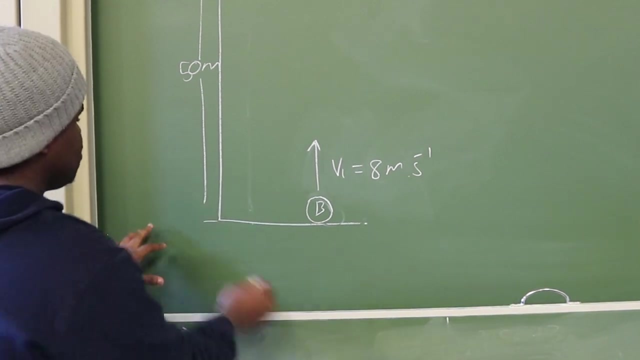 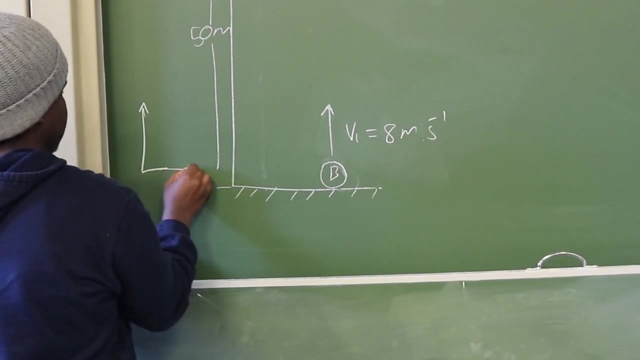 And for this one, say it was thrown upwards. it may be like 0.8 meters per second. So the first one, it was like 50 meters above the ground. So this is our ground here, this is the ground right. This is just our y-axis and this is just the x-axis, just to show the 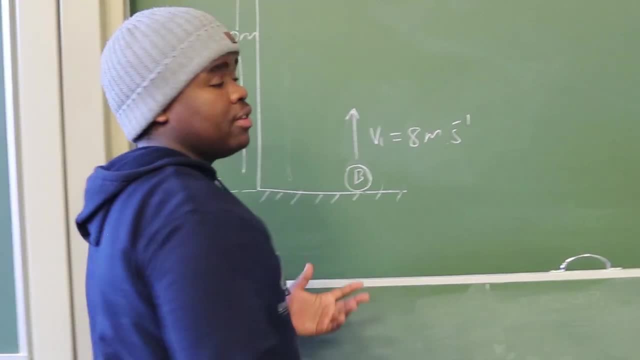 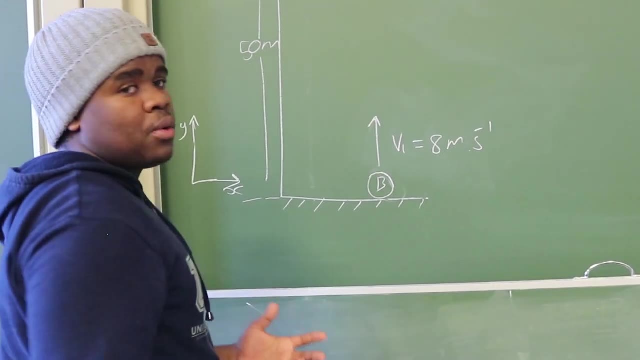 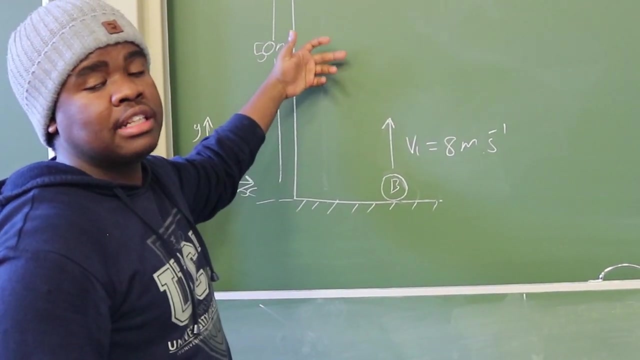 direction. Remember, we're dealing with vectors here. Velocity is a vector. it has magnitude and also a direction. so you have to take note of that. All right, so say the question. we're supposed to calculate the position at which these two balls meet above the ground. So how do we come about to? 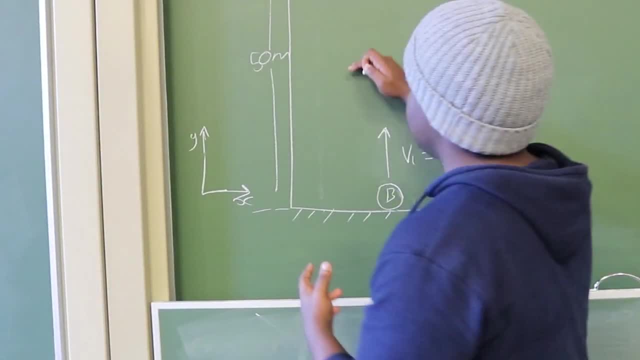 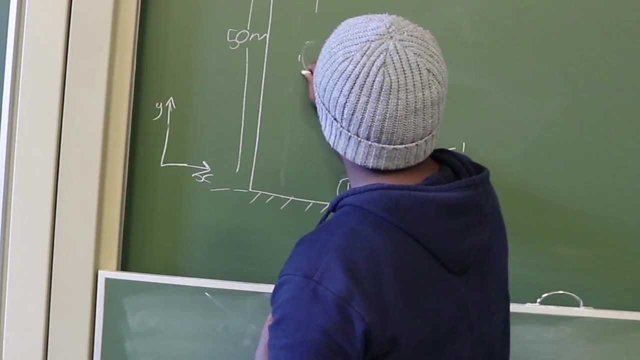 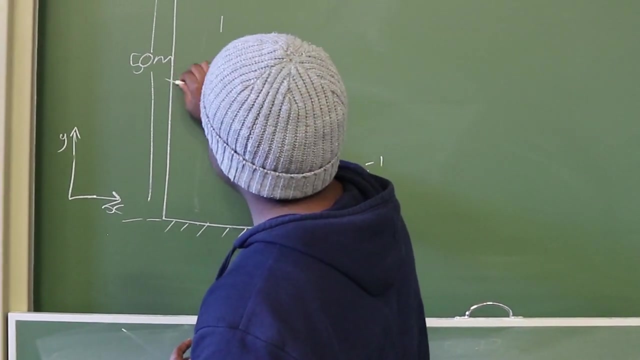 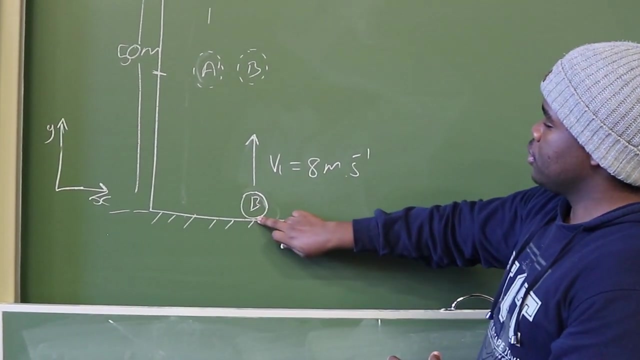 do that. So, firstly, if we were to calculate the position at which these two balls meet above the ground, maybe- say it's somewhere here, this is ball A, and then you have ball B. So you have two balls A and a ball B at some distance above the ground. We know that the time taken for this ball to just 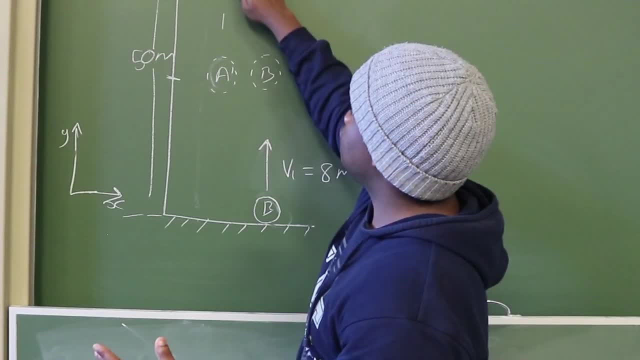 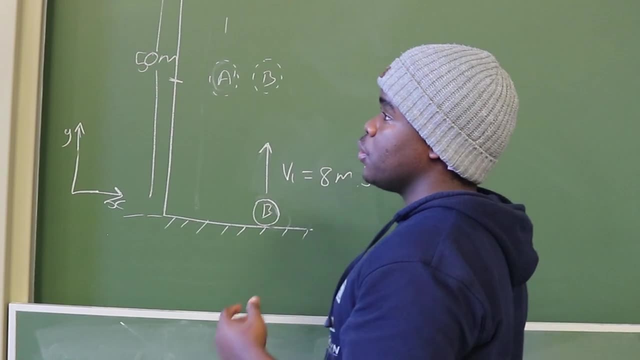 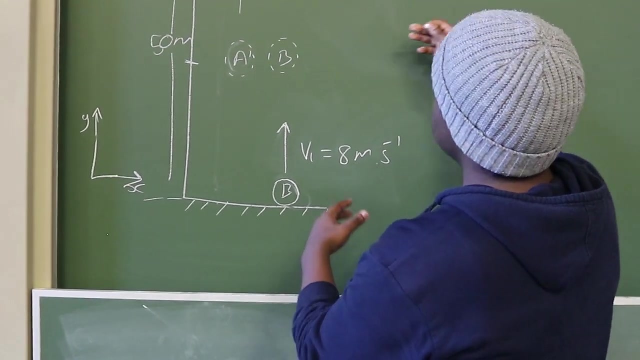 move from here today is going to be the same as the time taken for this one to move from here today, right? So we're just going to work with that, All right. so, firstly, we're looking for the position given the initial velocity, Okay so, and 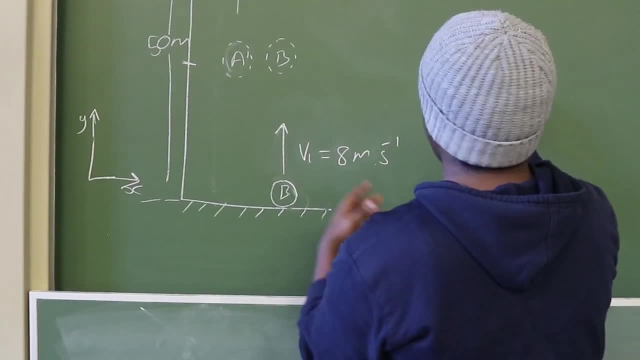 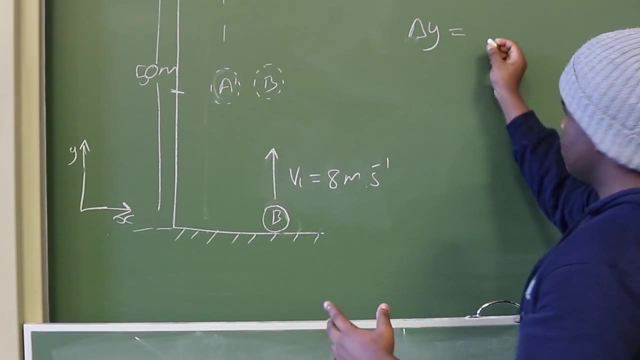 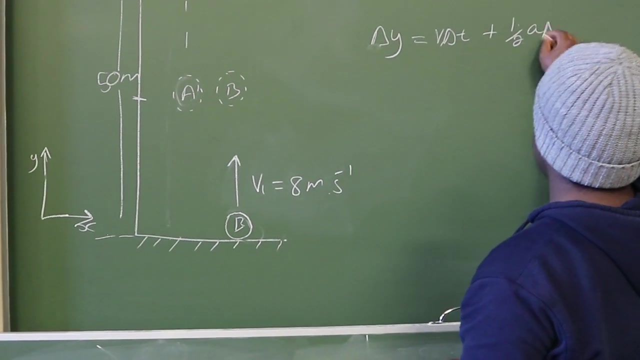 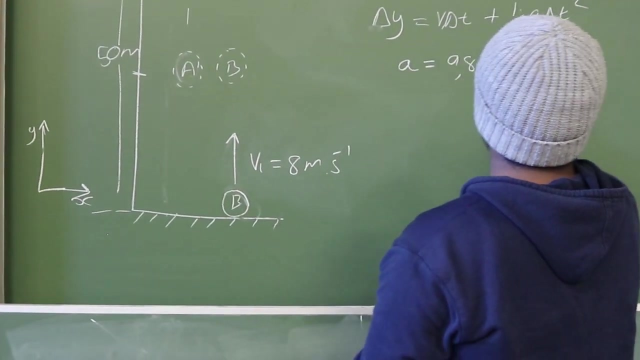 it, because you shouldn't just formula bash these kind of stuff. okay, so for this one you can use: the change in Y is equal to the initial velocity times, time plus half the acceleration delta. T, squared, where A is equal to 9.8 meters per second. 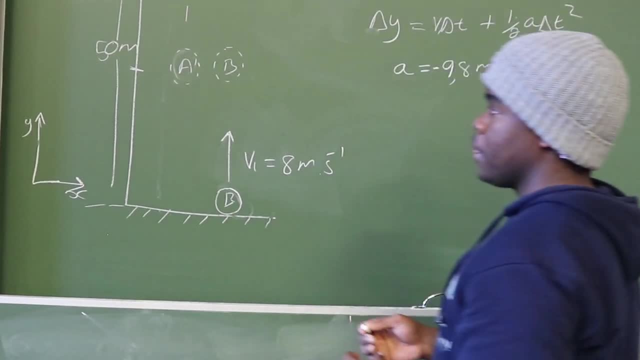 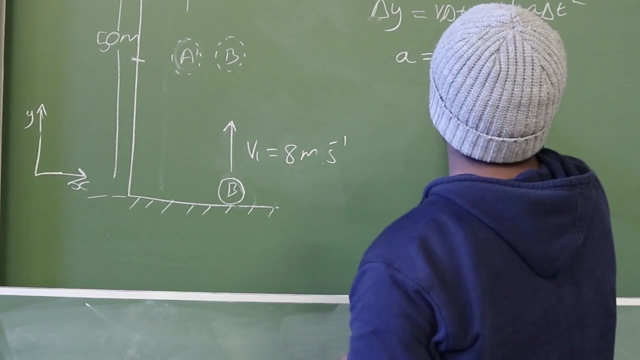 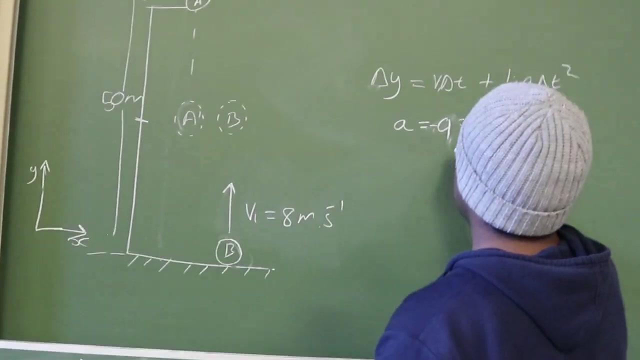 squared, it's negative. well, depending on which direction you take. yeah, it just depends on which side you take as a direction. but but, to be safe, always take the direction of motion as positive, right, just to make things easy. so you know, for this one it's just going up, so going upwards is just positive and going. 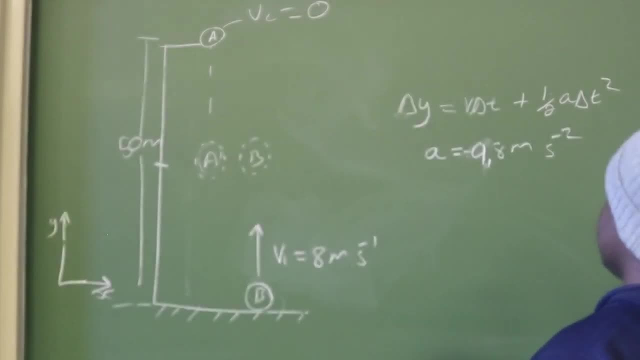 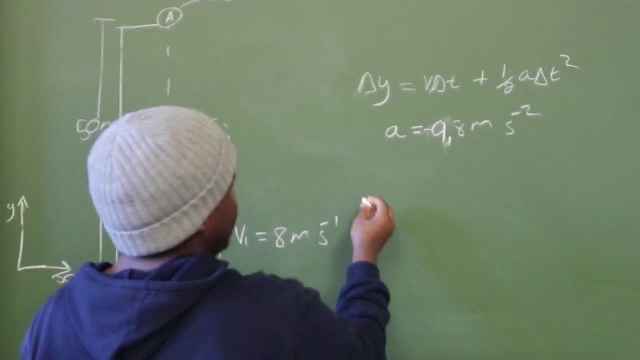 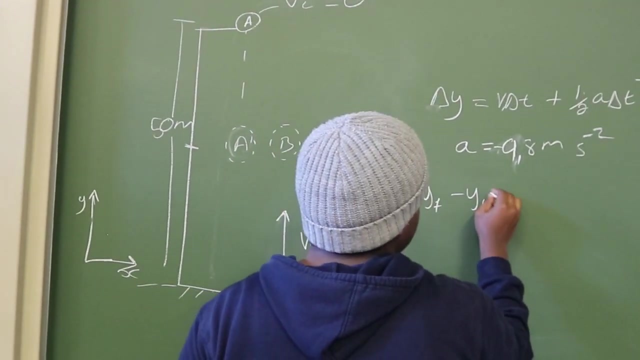 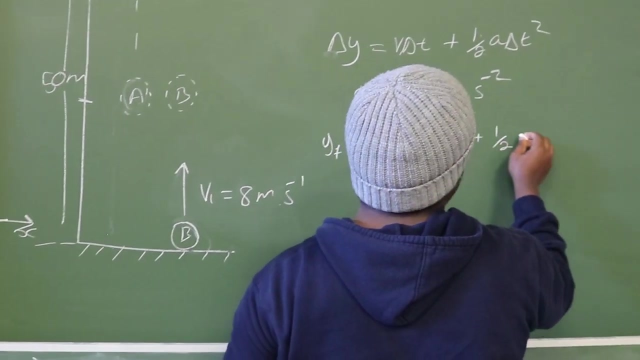 downwards is negative. you can even check from the axis here. cool, okay. so now we have to change for this one. okay, so the change is given by the position, which is final minus. the initial is equal to V letter T plus one over two, well, which is G, because it's just 9.8 and that's a T squared. right. then you know that your Y. 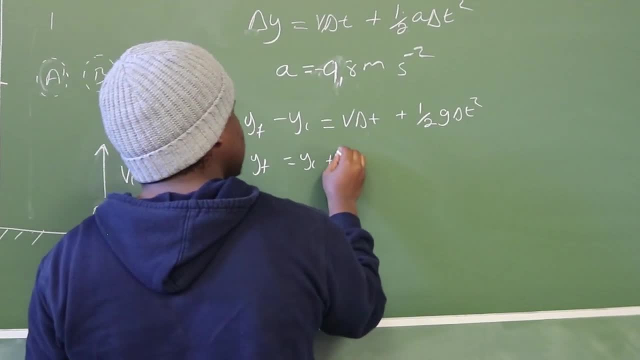 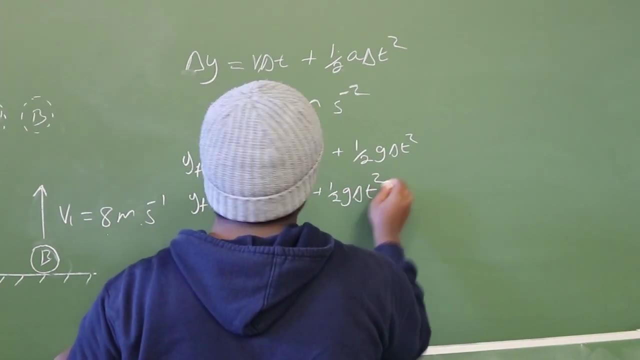 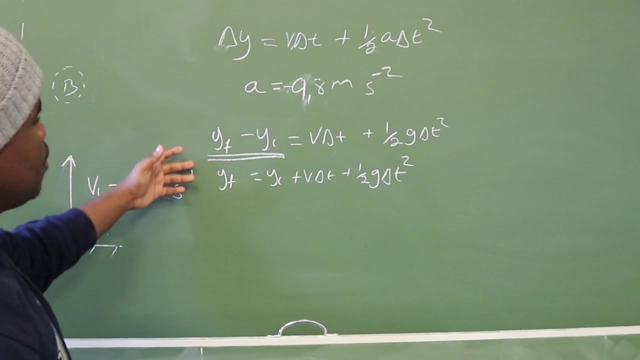 final is equal to the Y initial plus the initial velocity times delta T squared. t plus 1 over 2 g delta t squared. So I think this is the most important part when dealing with this kind of question. You should know that we're actually, when we talk about delta, 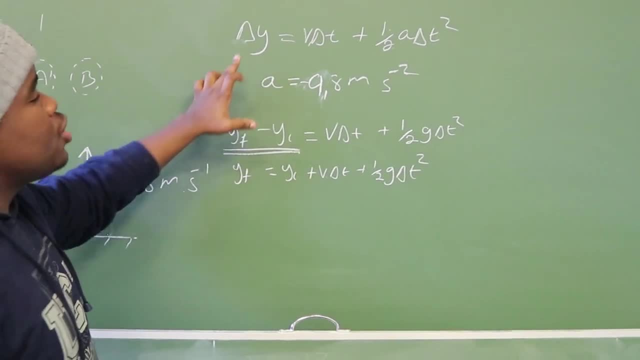 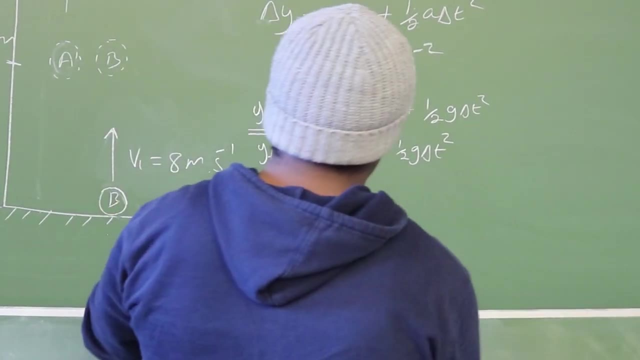 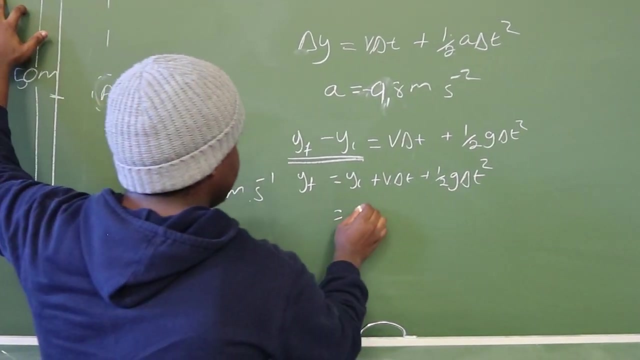 y, we're talking about the change, not the actual position. So in this case we're looking for the position, not the change. right, Cool, So now we can just calculate. So for this one, we know that the initial position was like 50 meters, and then the initial velocity. 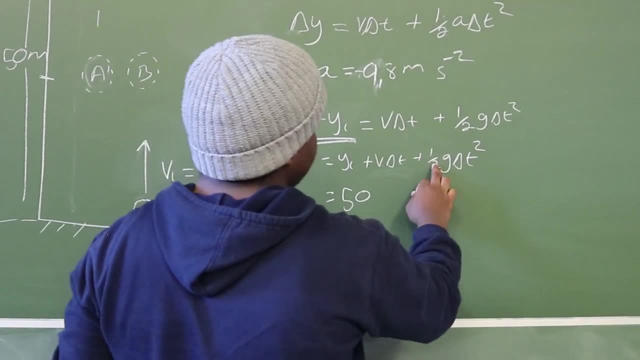 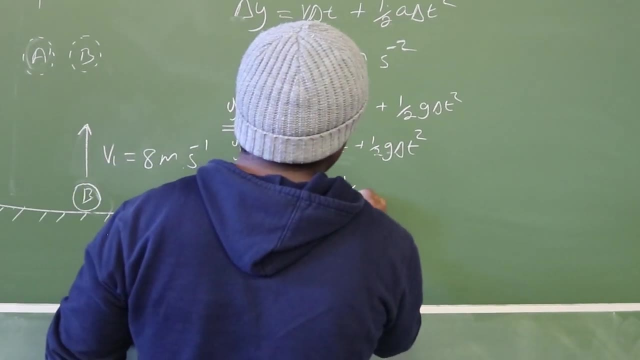 was 0, so this term just goes to 0, and then we have a negative, since g is negative, right? so it's just going to be negative. 1 over 2 times 9.8 delta t, so it should be like: 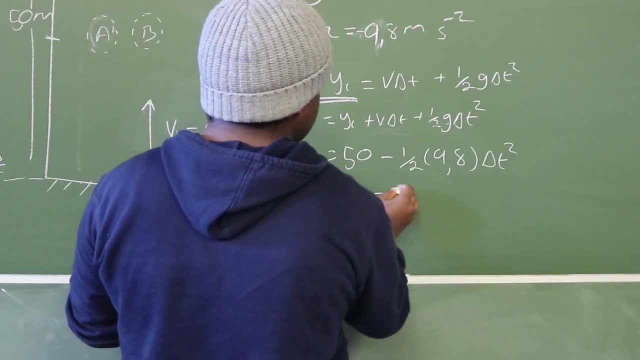 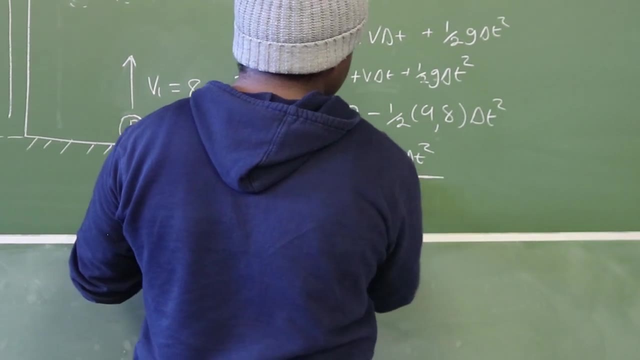 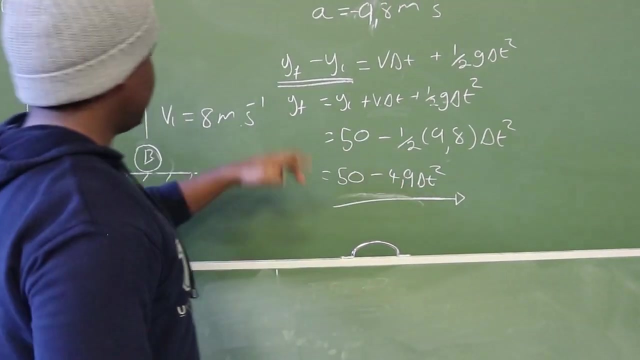 4.9, so we have like 50 minus. is it 4.9?? Yeah, I think 4.9 delta t: This is the position for this one at a certain time. t- We're going to have that, But we're. 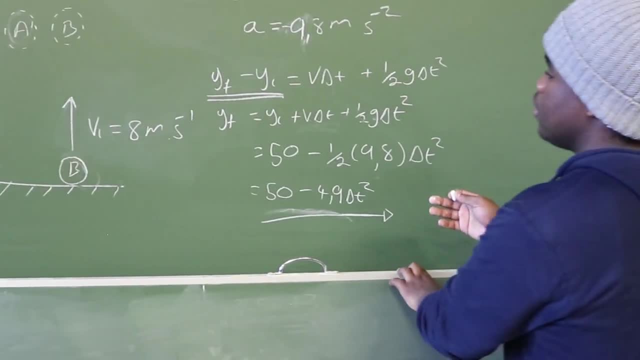 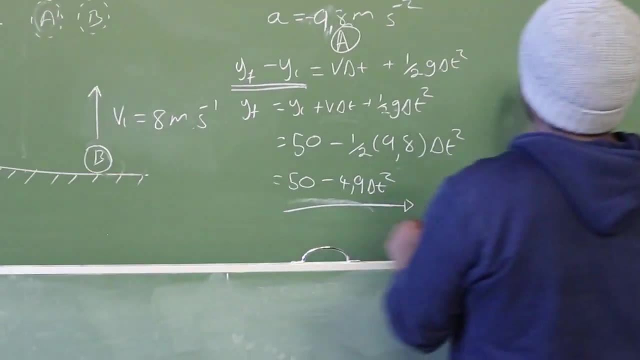 not done yet. So we do the same thing for the second ball, which is ball b. so let me just take here it's ball a, right. And then for ball b, we also do the same thing and also use the same formula. 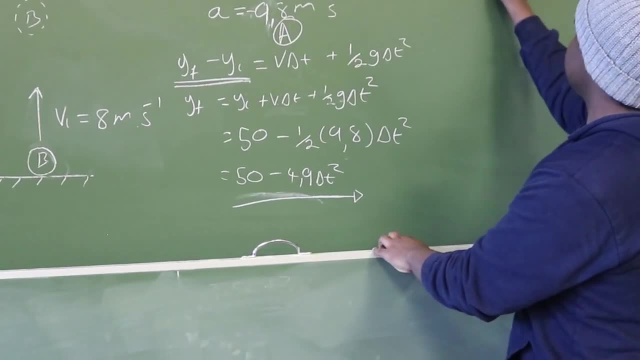 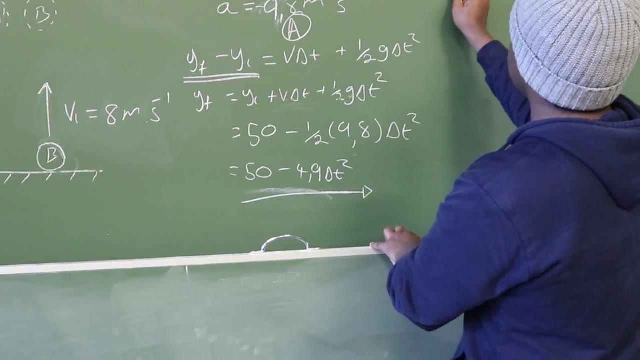 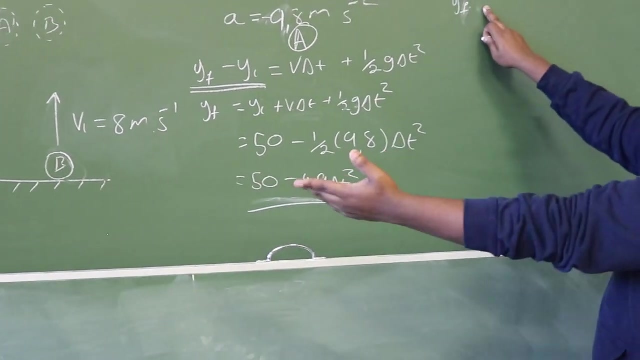 So we're going to have y. change in y is equal to initial velocity, delta t plus 1 over 2, a delta t squared where you change in y. so you're just going to have your y final. it's y final minus y initial and y initial is just 0, so the thing just goes to 0. Then 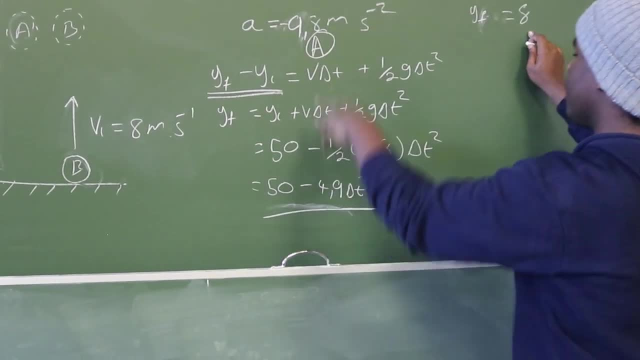 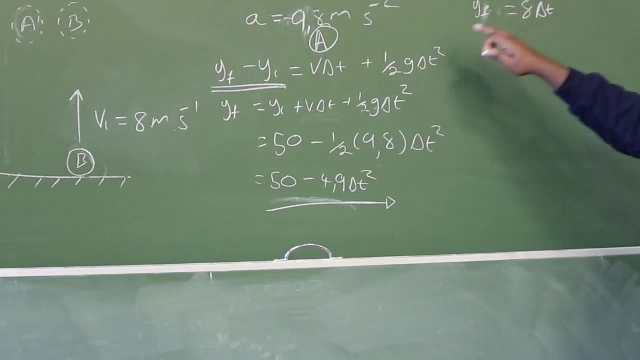 we have the initial velocity. it's 8 meters per second going upwards. it's positive delta t, then it's 1 over 2 times 9.8.. So we're going to have y bar equal to 2 over 2, and here we have y bar equal to 2 over 2,. 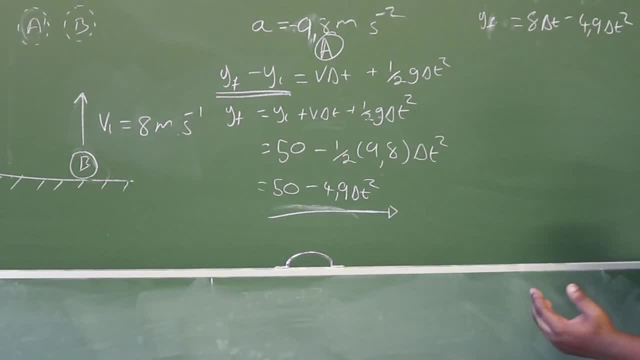 so now we're going to add y bar to 2 over 2 and add up and we'll get the value of 1 over 2.. So we're going to go ahead and put in in order to make that change. we're going to. 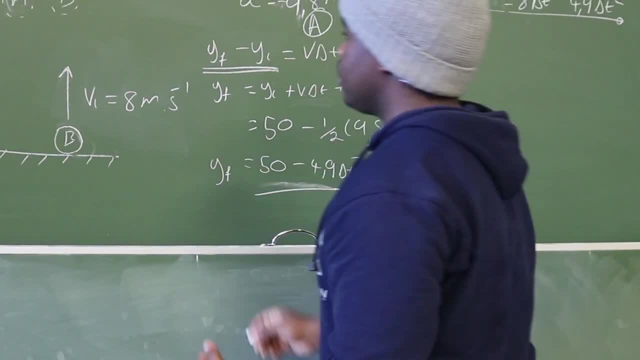 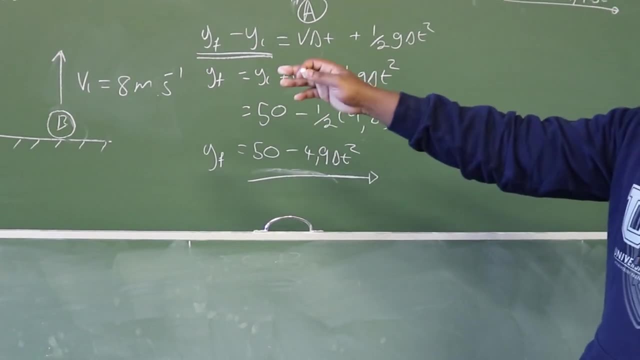 have, our y bar is equal to minus 2 over 2 and we'll add the y bar equal to minus 8 plus 2 over 2.. Now with y bar, we just have to take y bar equal to minus 9.8, which is just minus 4.9. 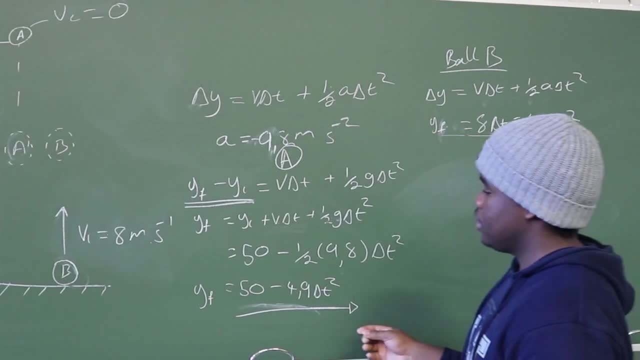 delta t squared. So what should you do from here? You just equate these two positions. Remember, the question was saying how to use the position at which these two, these two balls, meet above the ground. So now we have a problem. 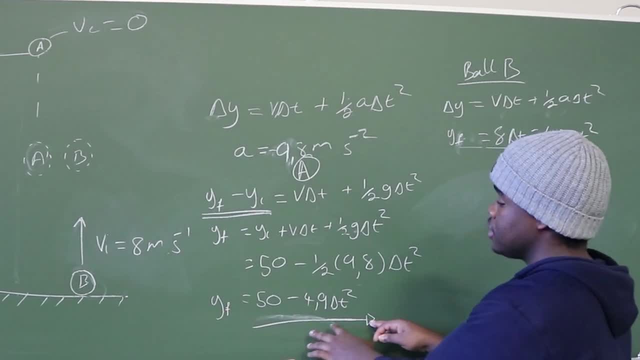 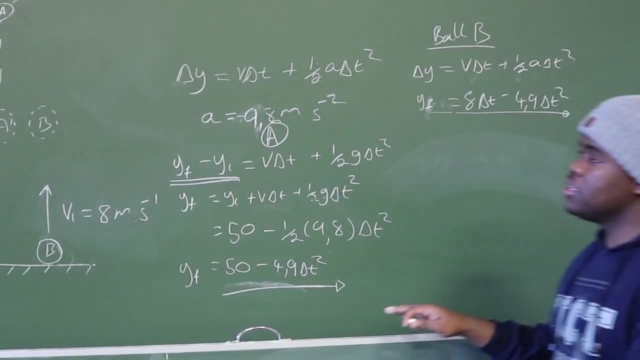 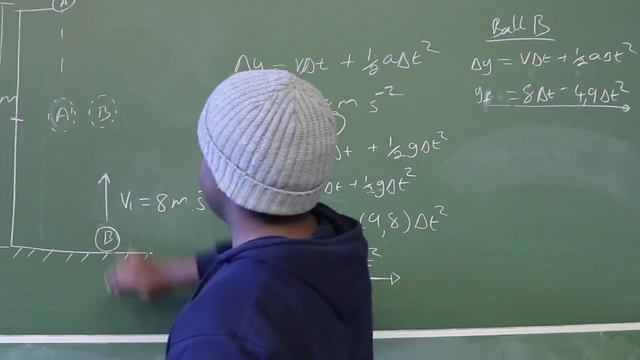 We have the position of block A as a function of time and we also have the position of block B as a function of time. Remember that we said earlier on in the video that when these two balls meet, it's going to take the same time for them to just cover different positions, obviously. 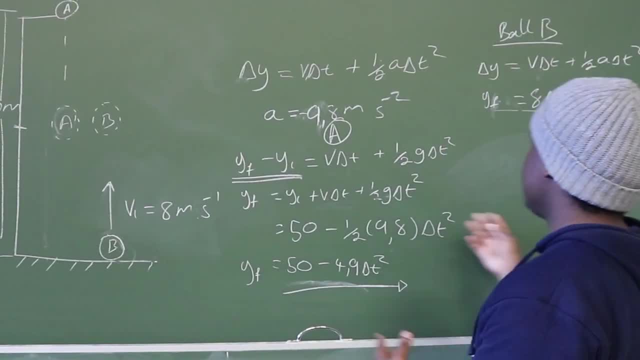 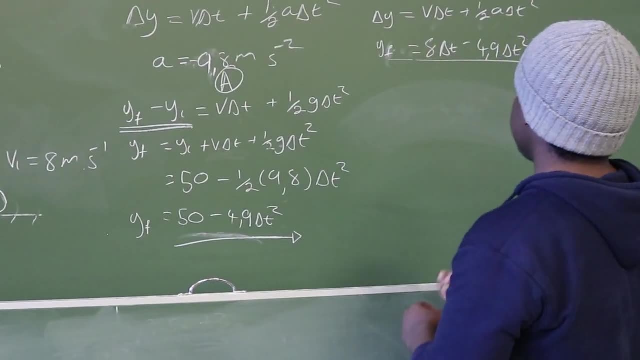 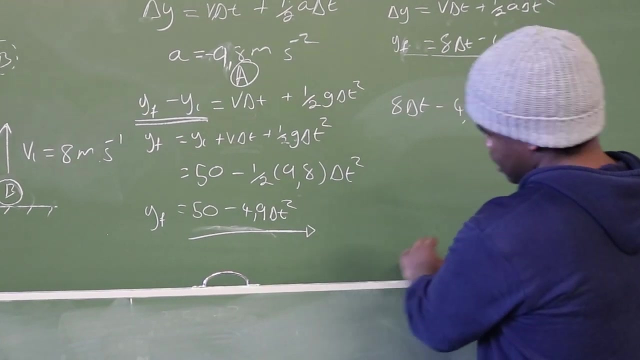 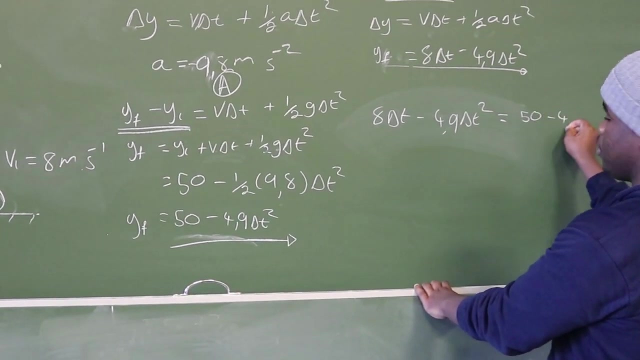 But then they're just going to get at this point at the same time, So the time is the same for both of these two blocks. So right now, what it's going to do, it's just going to equate these two equations. Alright, so we have 8 delta t minus 4.9 delta t squared, which is just equals. okay, fine, is equal to 50 minus 4.9 delta t squared. 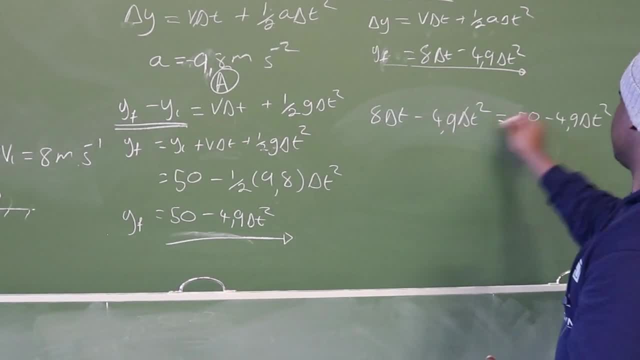 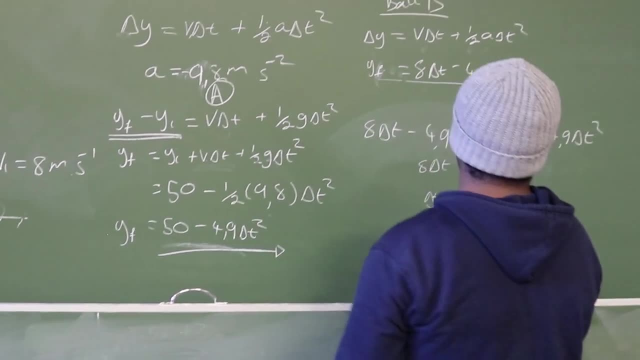 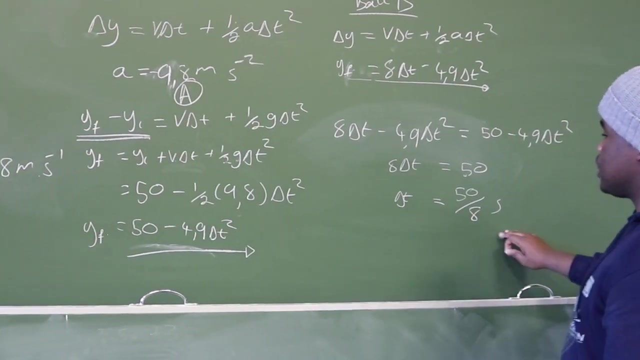 Oh, wow. so basically, just transpose this two, cancel out and you can get 8. delta t is equal to 50, fine, This is equal to 50. Divide by 8 seconds, right, And then from there, once you get your time, you can just take the time and substitute. 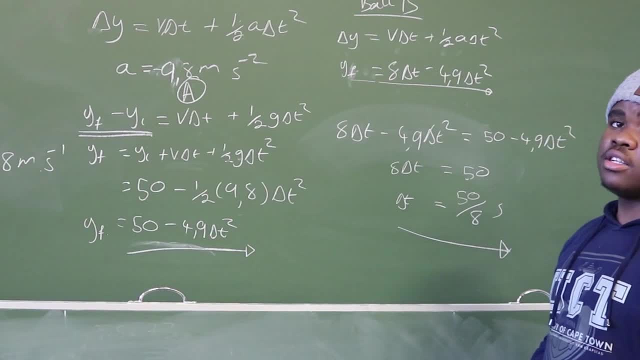 And with all of these equations, you should get the same answer. Thank you very much for watching and I'll see you in the next video. Bye, bye.